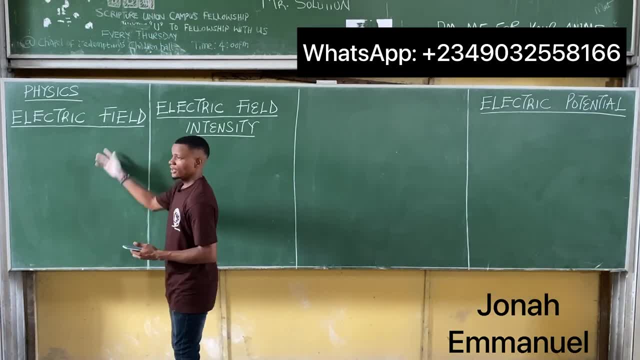 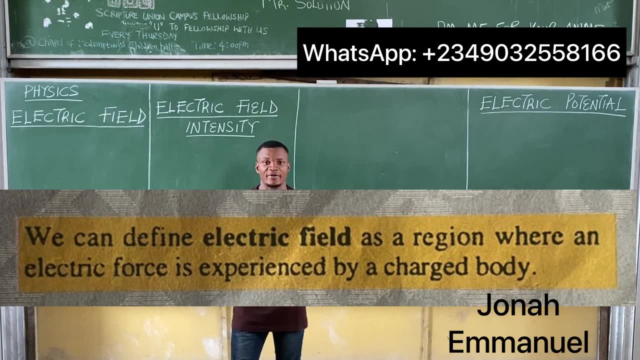 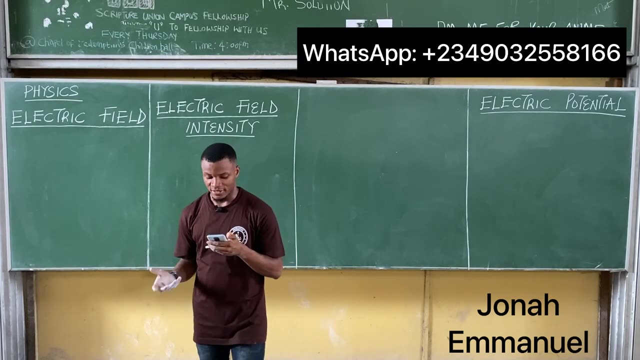 Now let's talk about the first one here: electric field. Electric field, by definition, is a region where an electric force is experienced by a charged body. This is what we define as an electric field. Now, usually, electric field is investigated by measuring the force on a small positive test charge. 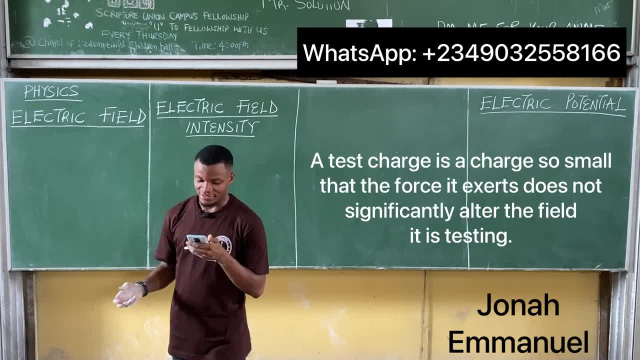 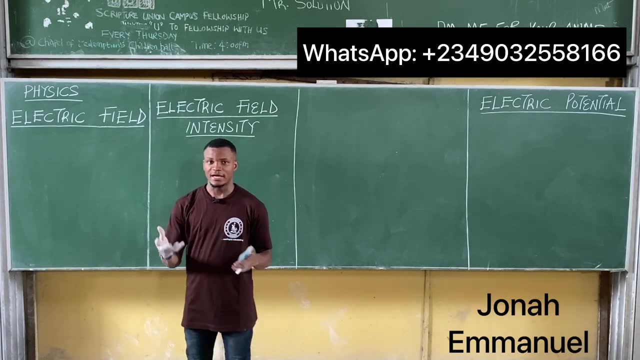 What's a test charge? A test charge is a charge that is so small that the force it exerts does not significantly alter the field it is testing. Now, if you want to draw a diagram for electric field, now we say we test or we experiment on electric field by using what is called a test charge, which I have defined earlier. 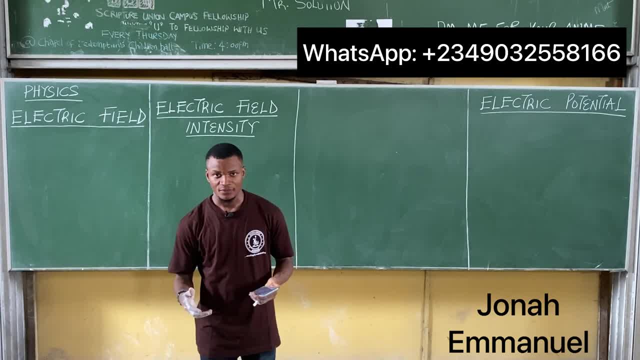 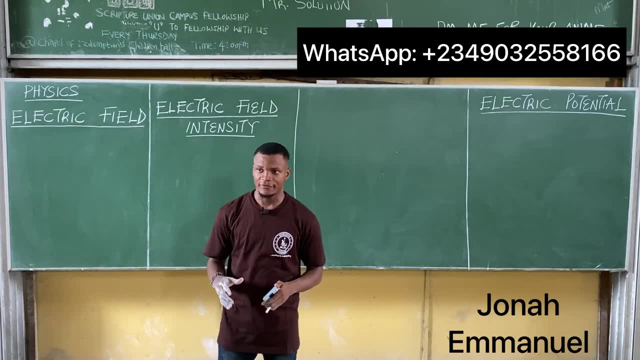 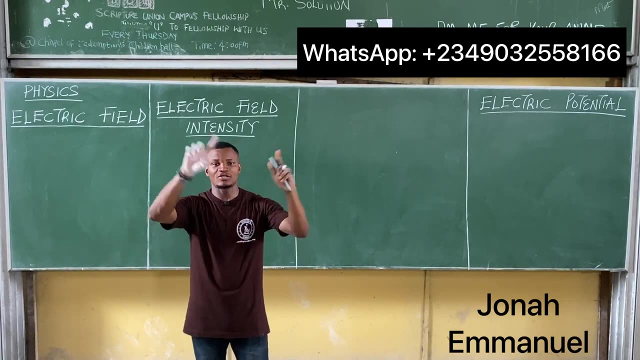 Now this is what we call electric lines of force. For instance, if I have a positive charge and a negative charge being brought together, we say from the first law of electrostatics, there will be an attraction. This attraction causes an electric field to be built around them and this electric field can be represented diagrammatically using what is called electric lines of forces. 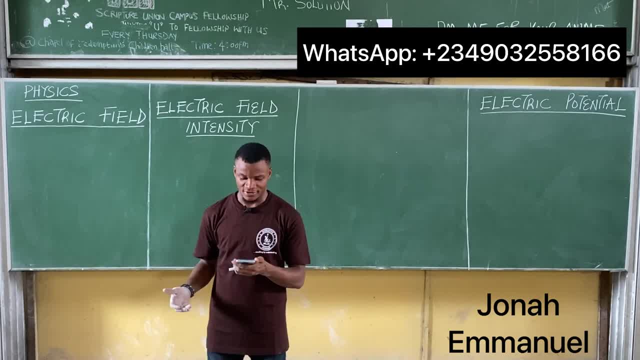 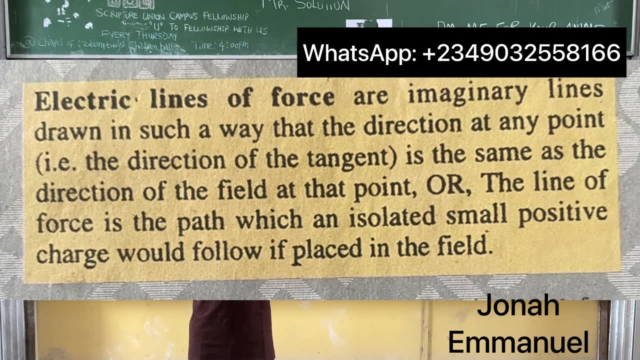 Now, what are electric lines of forces? By definition, they are electric lines of forces. Electric lines of forces are imaginary lines drawn in such a way that the direction at any point, that is, the direction of the tangent, is the same as the direction of the field at that point. 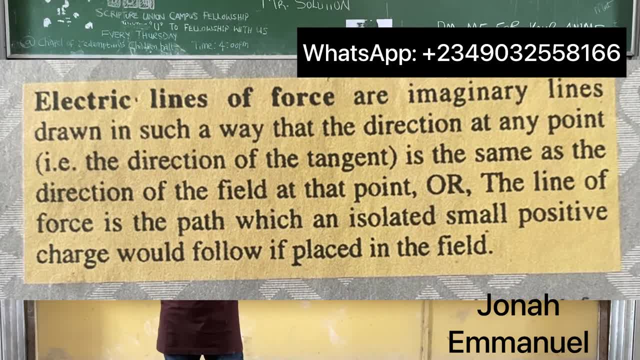 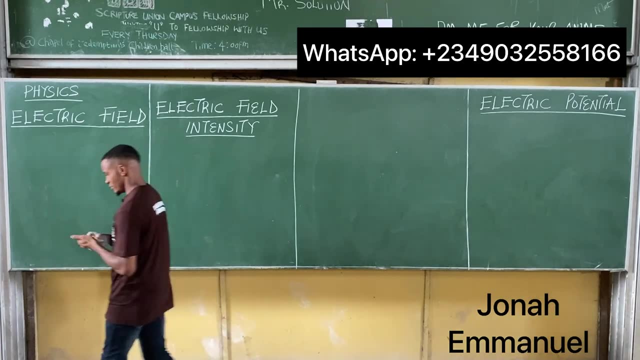 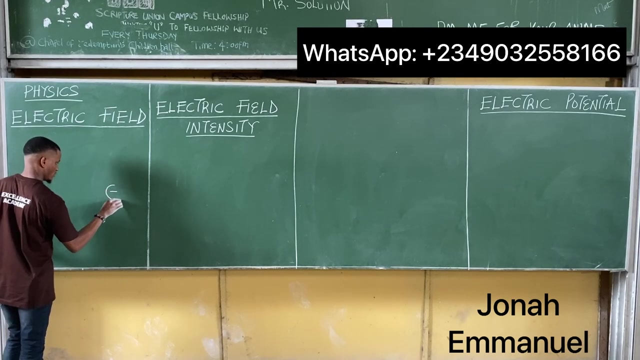 We can define electric lines of force as the path which an isolated, small positive test charge would follow if placed in the field. That's how you define the idea of electric field. Now, literally, if I have a positive and a negative charge, now we say there would be an attraction of this manner. 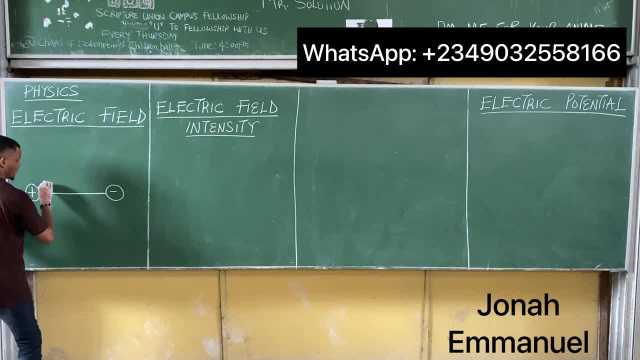 This to this, this one to this, This to this. Have this one going this way, Have this one going this way. Alright, so say, your direction is that to move from positive to negative? that's a direction, Alright. so this is like a diagrammatic representation of an electric field. 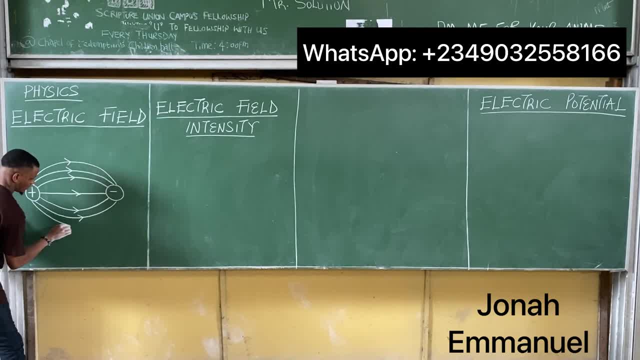 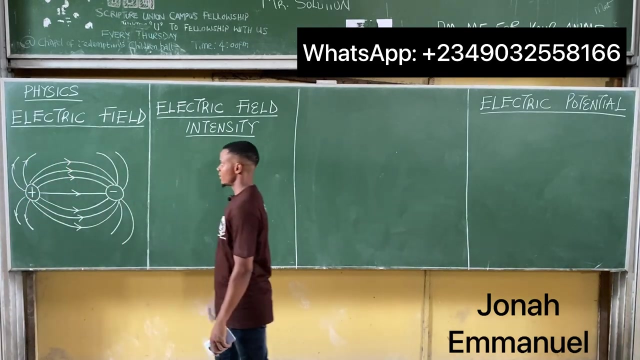 Okay, you have this. Take this one off like this. Have this one going this way, Alright, so look at this. This is what an electric field looks like. Alright, so this is how you represent an electric field in a diagrammatic form. 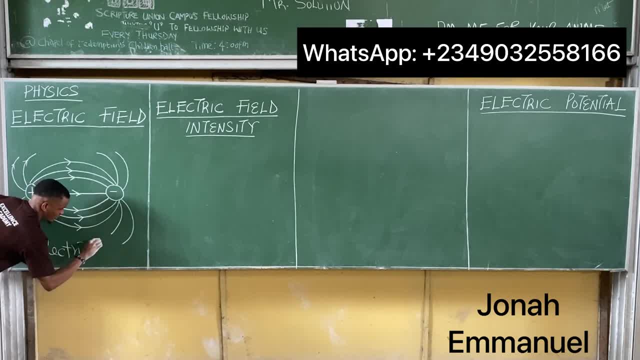 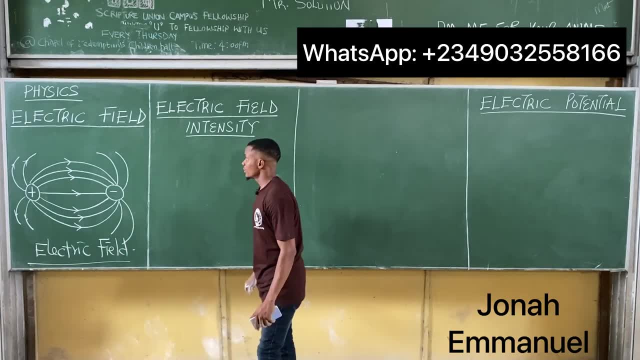 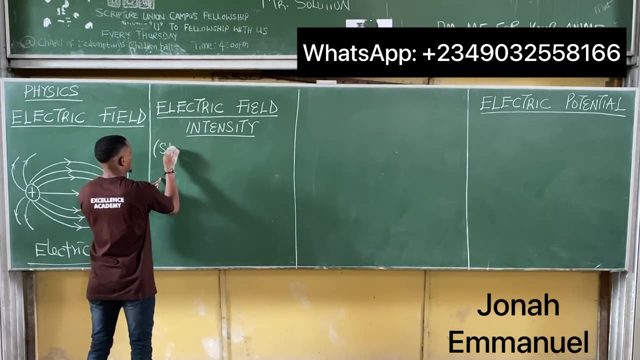 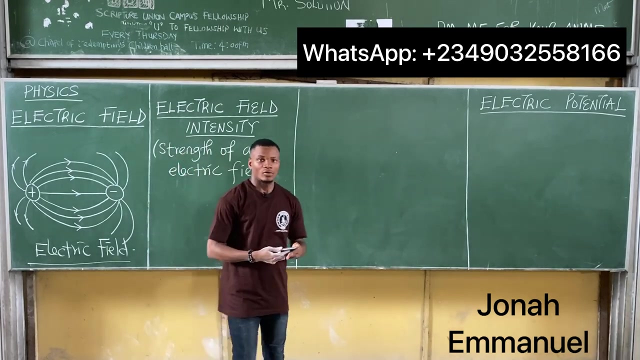 This is an electric field, Alright. so you have this Alright. so that's the first one electric field. Let's go to the next one here: electric field intensity. Electric field intensity is also called the strength or and electric field. 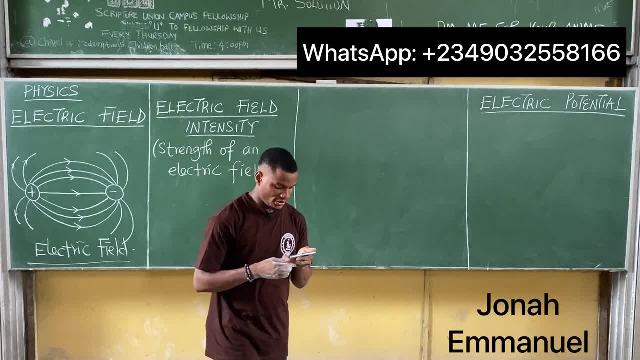 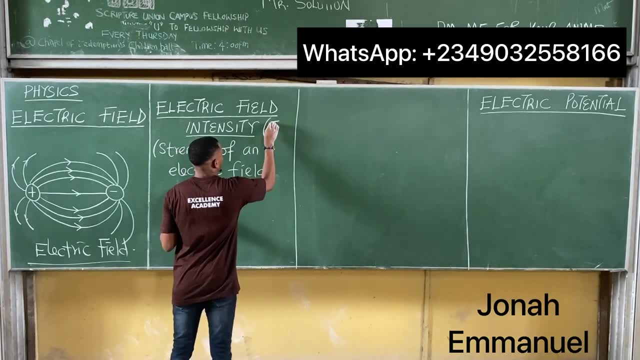 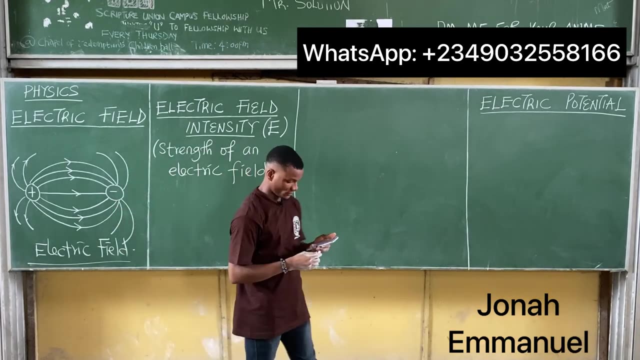 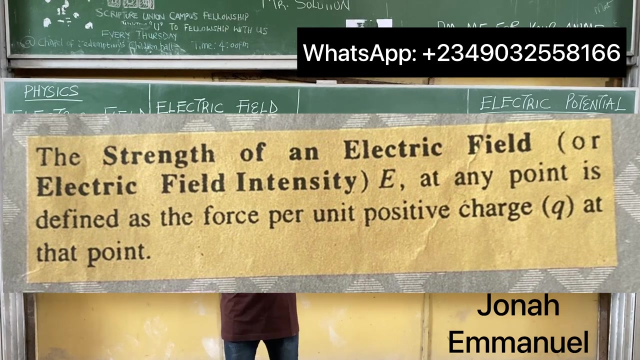 An electric field. By definition, the strength of an electric field or electric field intensity is E- Alright. this one here is E- Electric field intensity or the strength of an electric field- Alright. by definition, the strength of an electric field at any point is defined as the force per unit positive charge cubed at that point. 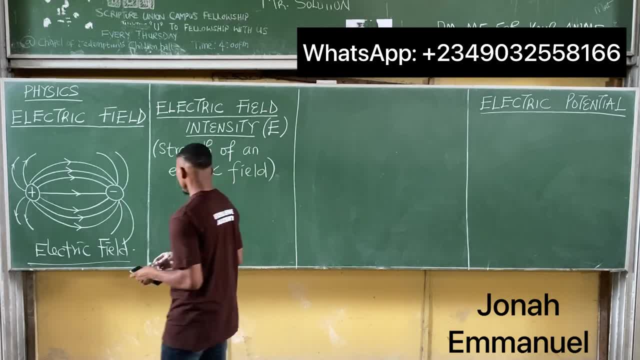 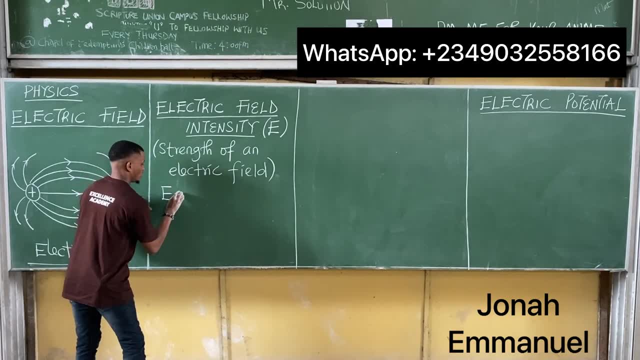 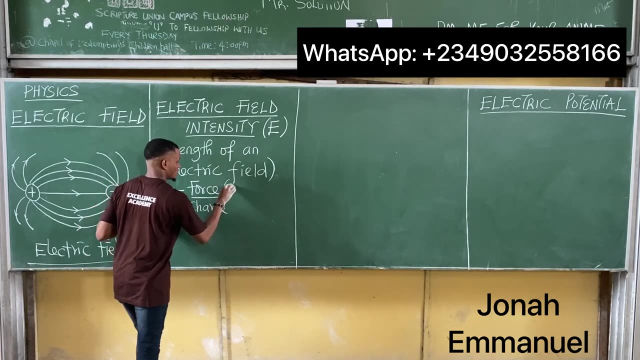 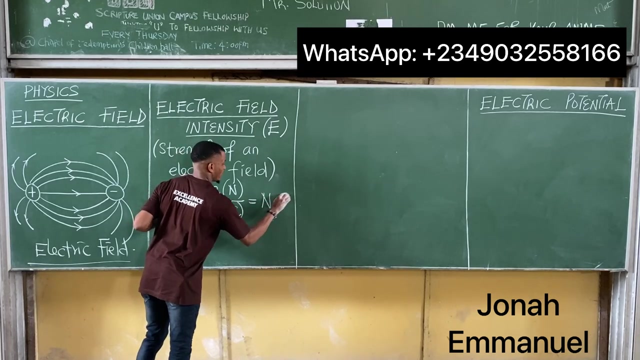 So it's simply force per unit charge. So if we want to get this in mathematical form, we say: mathematical E is equal to force all over charge, Force in Newton, charge in coulomb. So the SIU is Newton per coulomb. 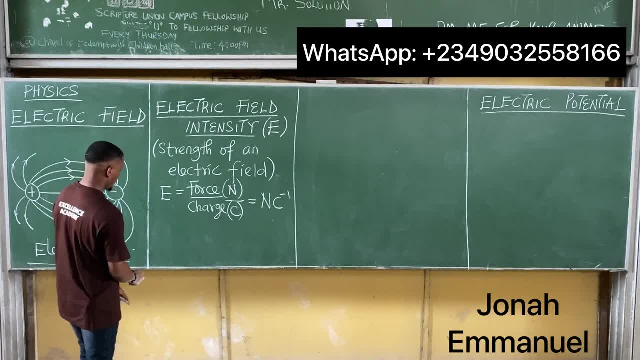 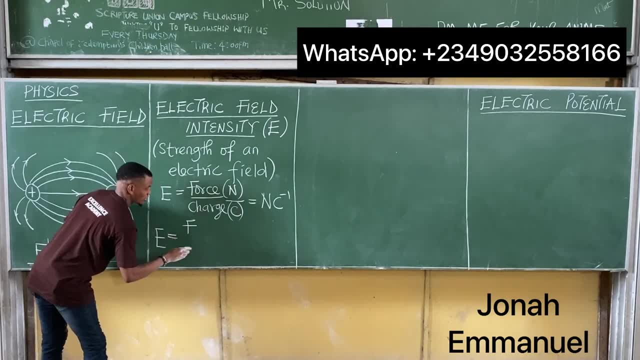 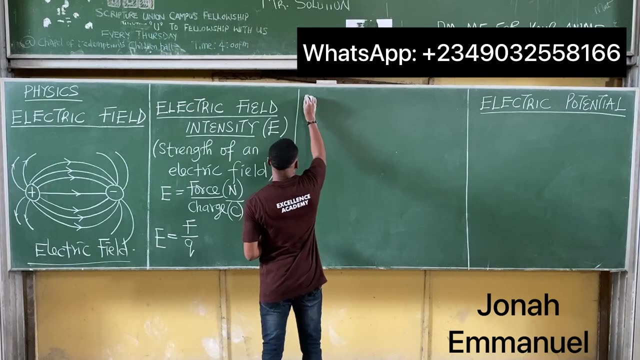 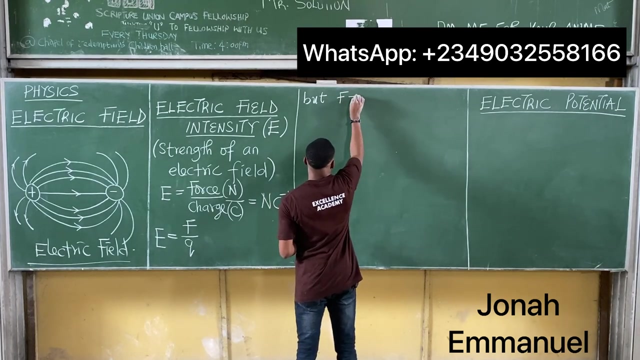 Electric field is measured in Newton per coulomb. So in a broader view we say E is equal to F, all over charge into Q measured in coulomb, But, but, but, but From Colu's Law we said force F is equal to K. 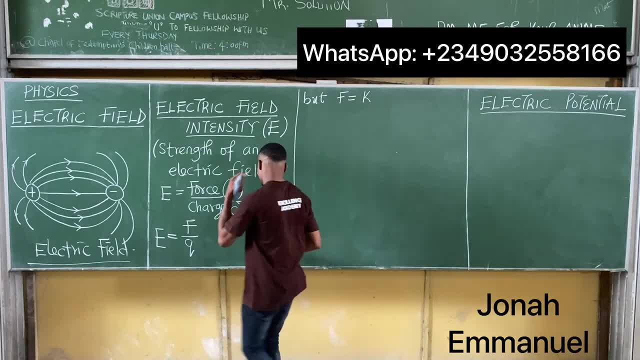 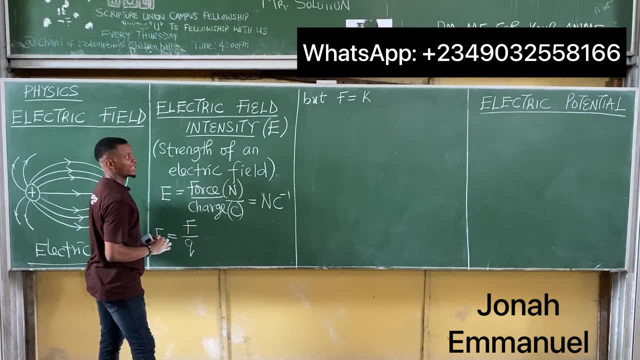 Let's say the force is F in broad bar. We said a positive tension, this one here. And let's say another force, Without using the idea of Q1 and Q2. We can still use the forces here as capital Q- This- and small q, that is this: 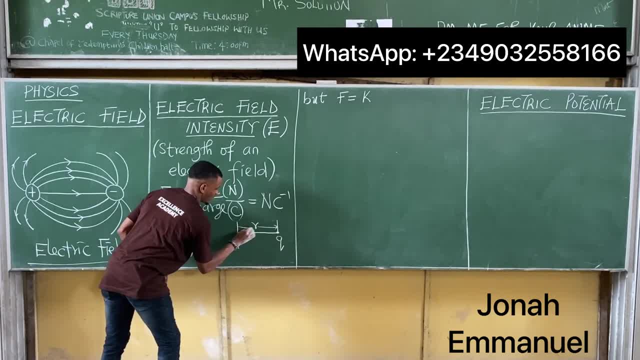 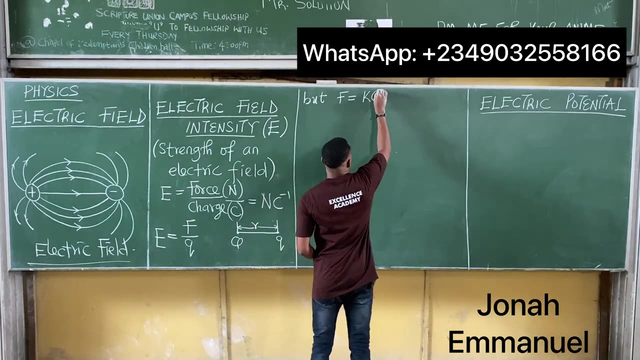 The distance. here is I Still the same concept. So instead of using Q1, Q2, I'm using the capital Q and the small q For this one here, from Colu's Law, The force of attraction becomes K, Q, Q all over R squared. 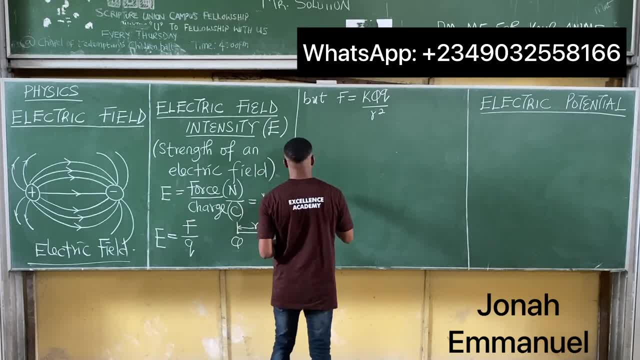 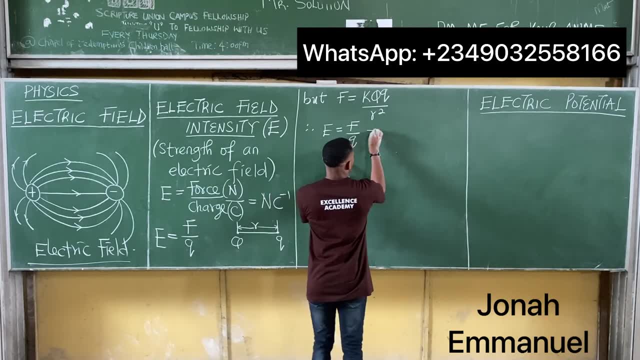 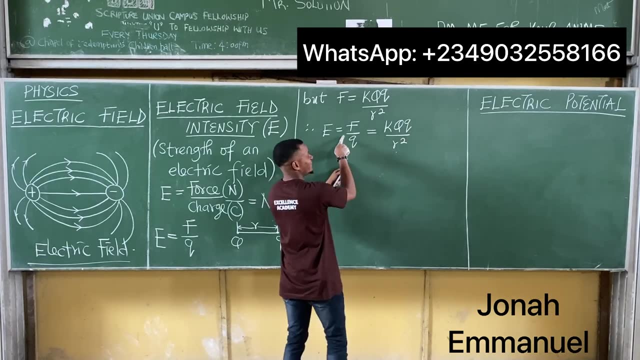 From this whole set. So therefore we can say that E is equal to F, F all over Q, That would be equal to F. The value of F is K, Q, Q all over R. squared Divided, so divided by, We have Q here, so we have this Q. 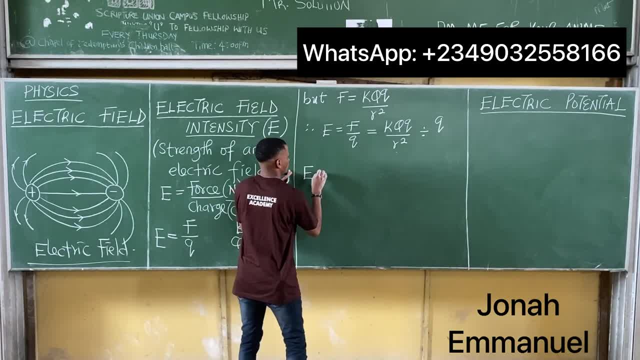 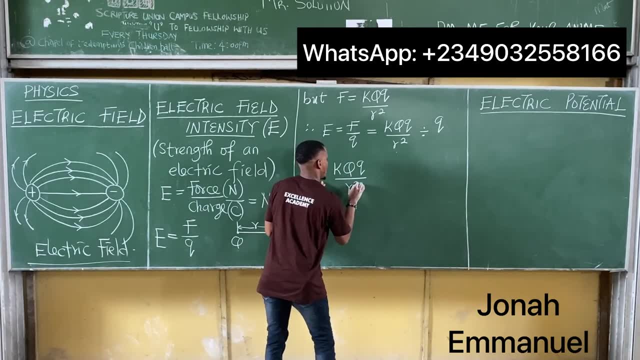 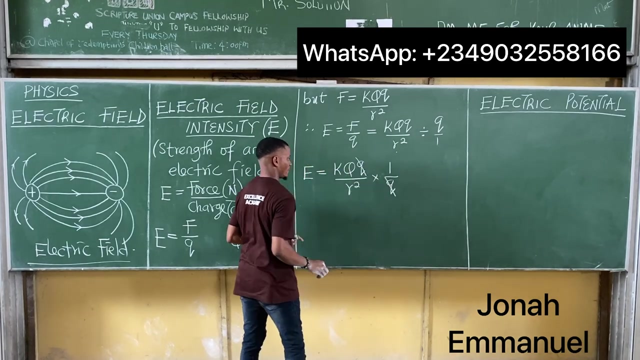 So here the electric field intensity E Is equal to K, capital Q, small q. All over R. squared times. Change up the term because this is divided by Q1. Same thing. So change up the terms and then invert To become 1 all over Q. From here now, Q cancel Q. 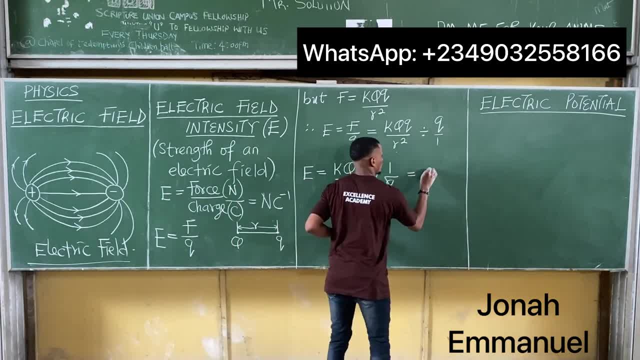 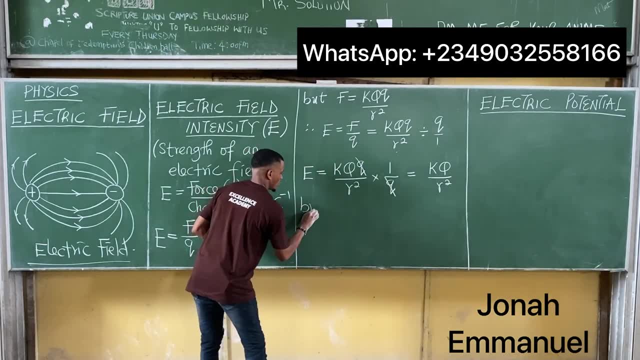 So E is equal to K capital Q All over R squared. So you have this, But we said K is equal to 1 all over R, 4 pi E naught. So hence E is equal to, E is equal to K, That's 1 over 4 pi E naught. 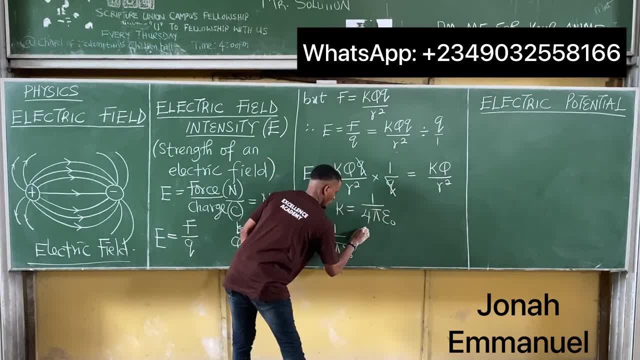 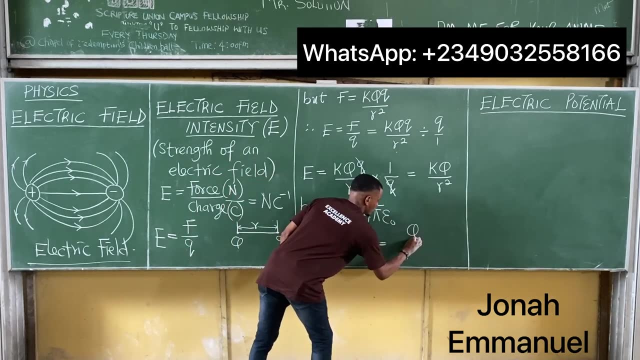 Times Q all over R squared, Alright, so K Q all over R squared. If I combine this, The electric field intensity E E is equal to 1 times Q. That's Q all over this 4 pi E naught R squared, So this becomes the. 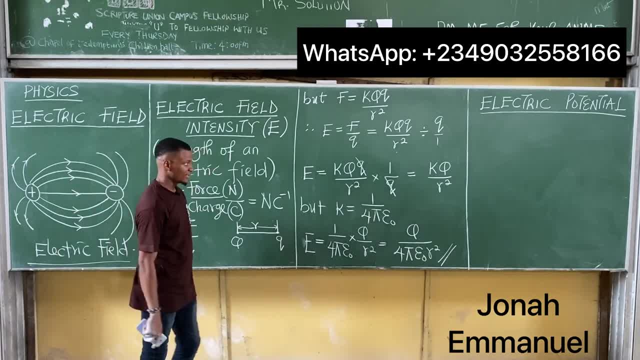 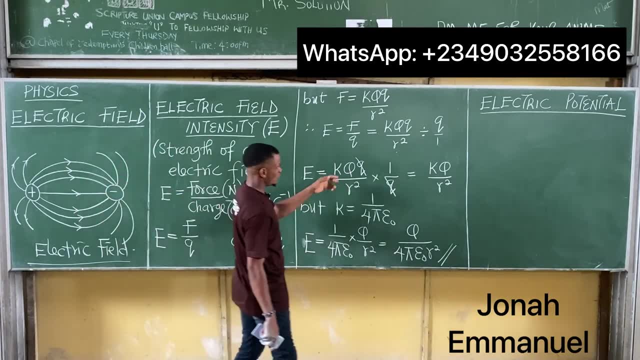 Formula for electric field intensity. Either you use the first one, Which is L by Q Thin value, Or the second one here, Which is K, Q over R squared Thin value, Or the third one, Q all over 4 pi E naught R squared. Whichever one you have, 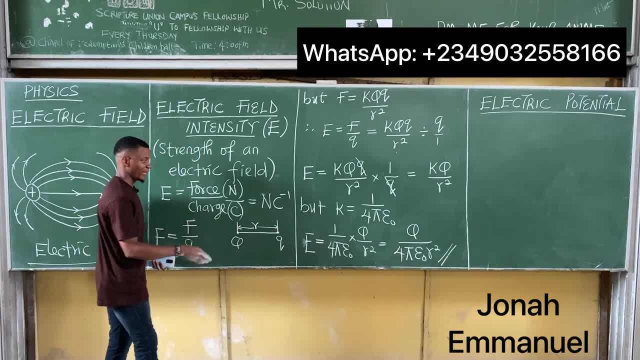 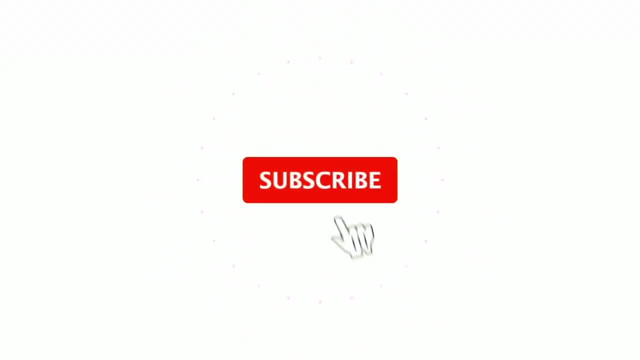 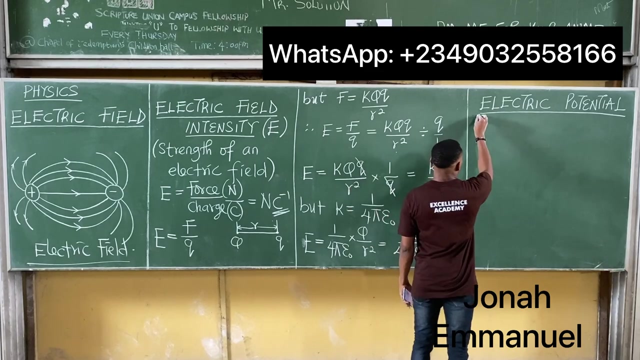 The correct answer. And for each of these, The SIU still remains Newton equality. So this is how This is the idea of Electric field intensity. Finally, let's look at Electric potential. So now let's look at Electric potential. This one is represented by V. Alright, So electric field is E. 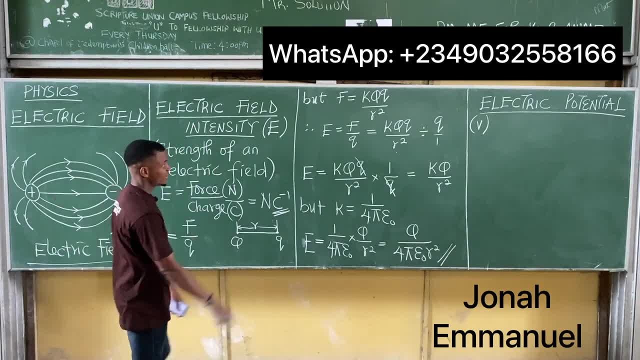 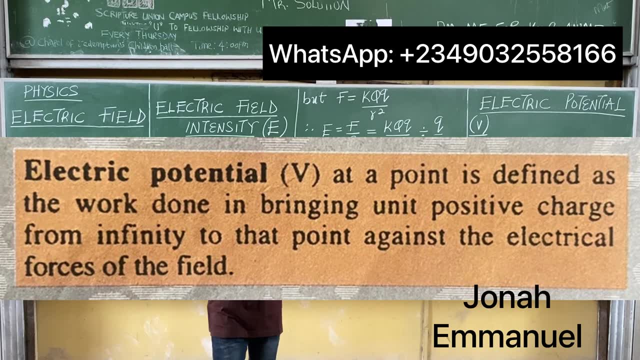 Electric field. intensity is E. Electric field is this. Electric potential is V. So what then, is Electric potential? Electric potential V At a point Is defined as The work done In bringing Unit, Unit Possibility, Charge From infinity To that point, Against the electrical forces Of the field. 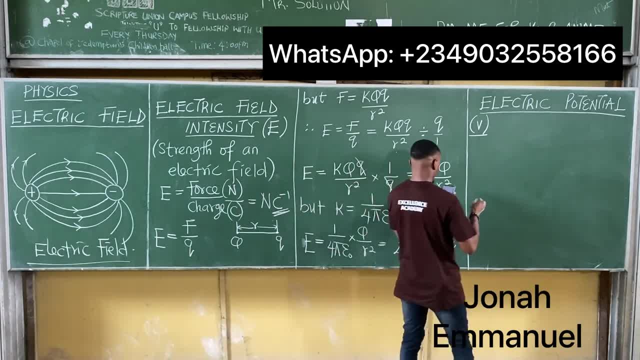 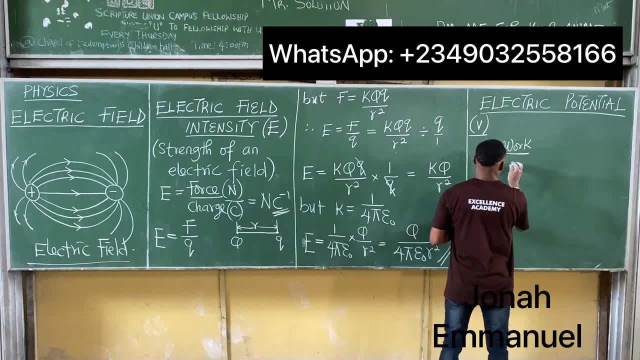 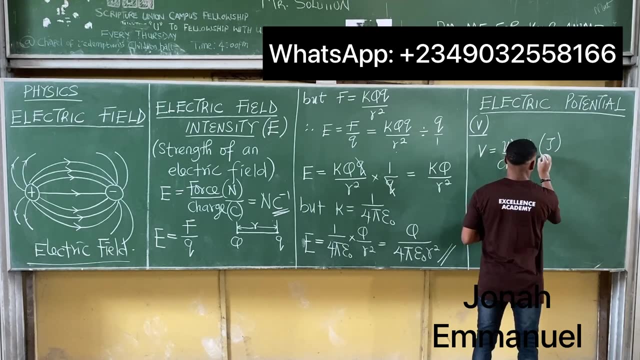 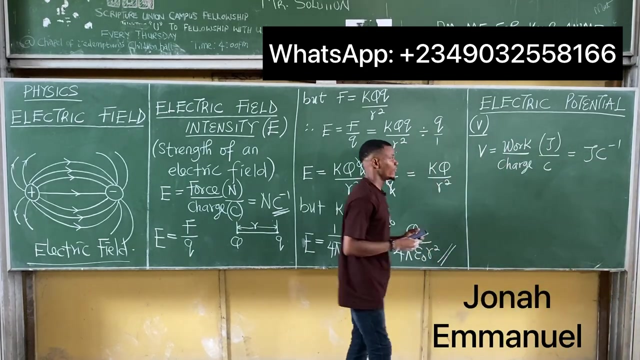 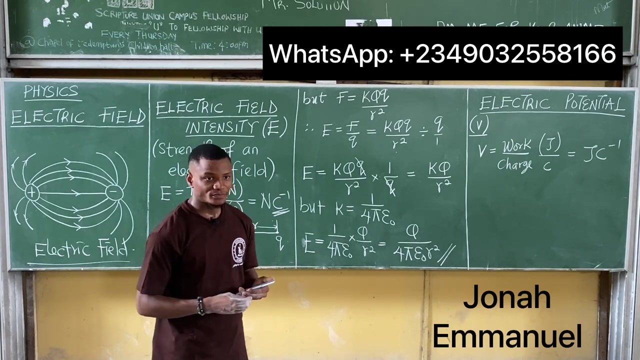 Alright, Mathematically, Electric potential V Is equal to Work done, Work All over charge. Work, of course, Is measured in Joule Charge With cooling. So SIU is Joule With cooling. That is the SIU for Electric Potential. Now This is one concept. Another concept is this: 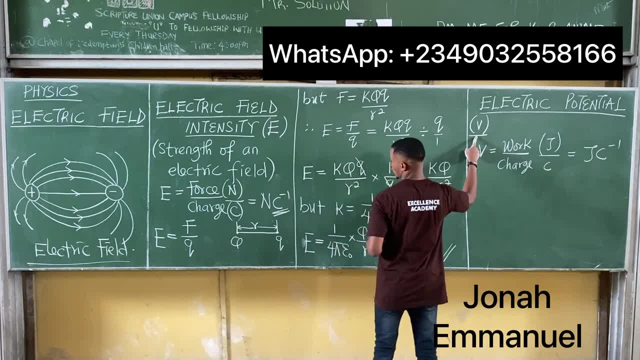 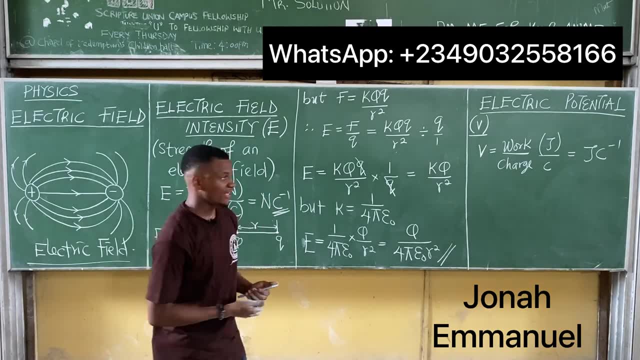 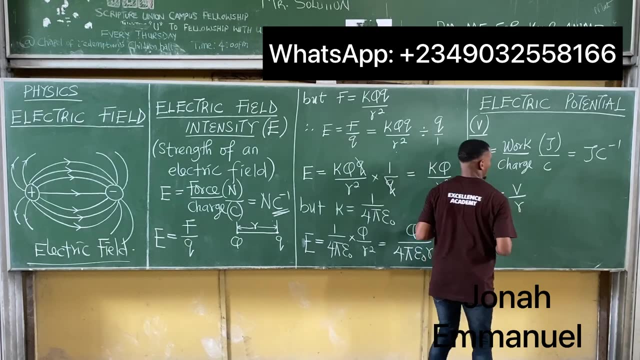 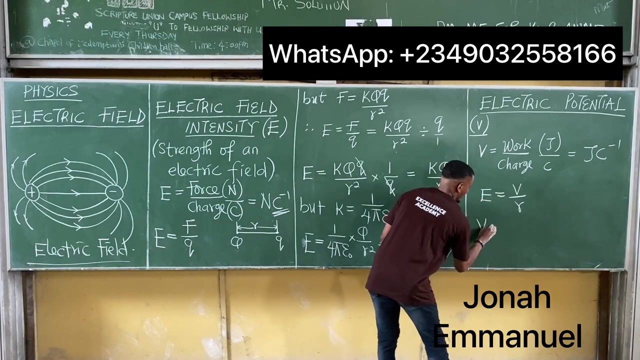 In trying to relate Electric potential To Electric field intensity. The relation between Electric potential And Electric field intensity Is given by: E Is equal to V All over I. So With this one here We can see that The electric potential V Is equal to The product of The electric field intensity. 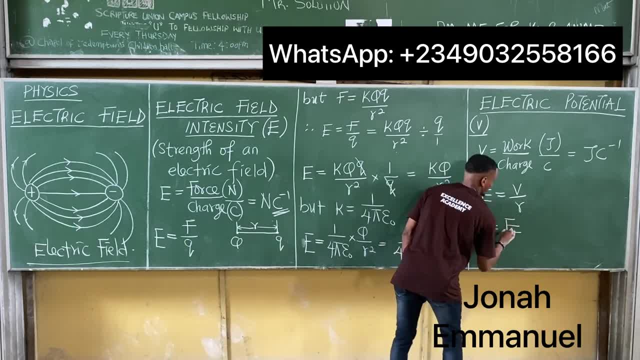 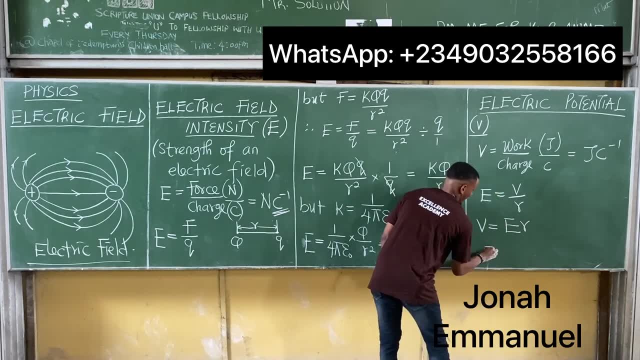 Electric field intensity E And The distance Of separation Or distance Given, That is R. From this We said: I like to keep The intensity. The SIU is Newton per column Or Newton per column. So Newton Per column Multiply Distance In meter, So that is equal to Newton Meters. 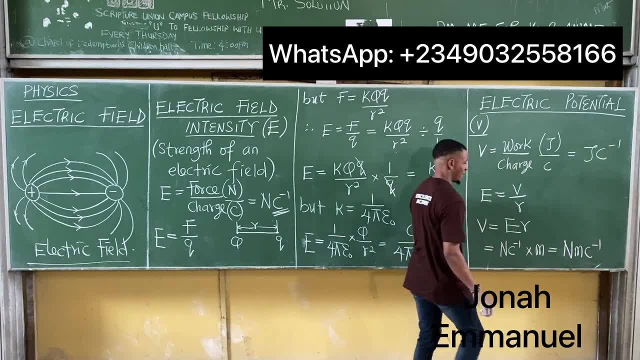 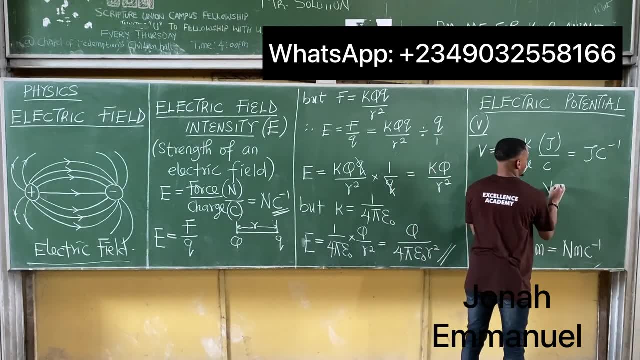 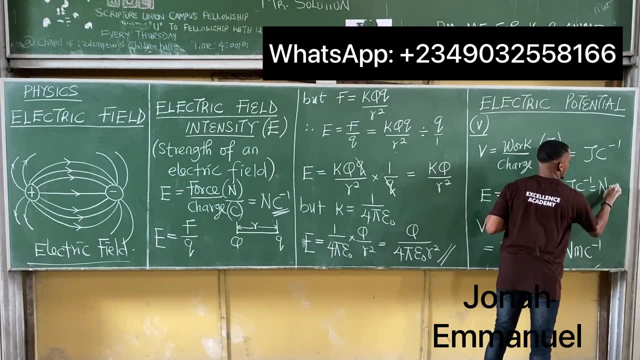 Come here Meters Per column Per hour. So the SIU of electric potential Is Newton meter per column. That means Electric potential V Is measured In terms of Joules Per column. Is also Equal to Newton Meter Per column. So Any of this Is the SIU Of. 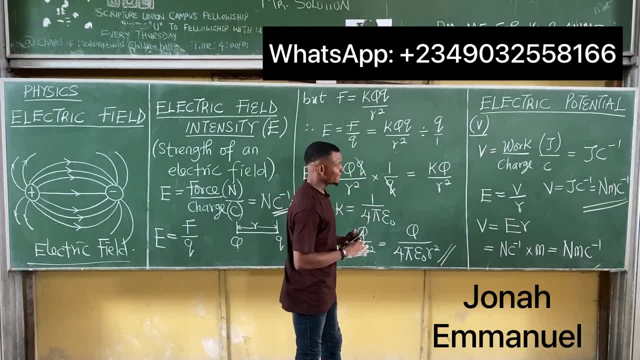 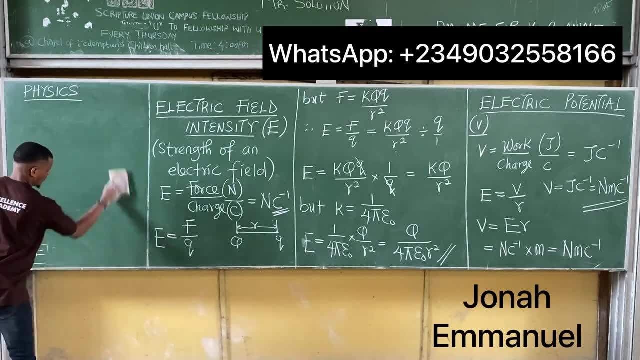 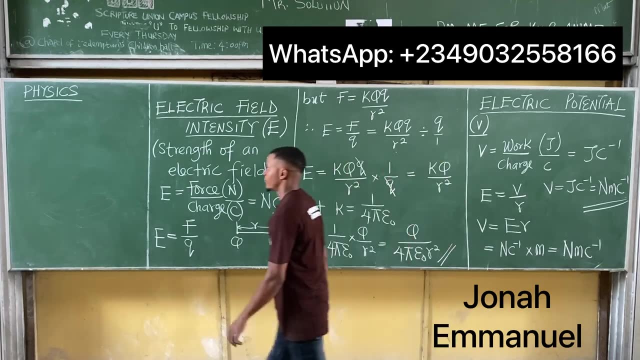 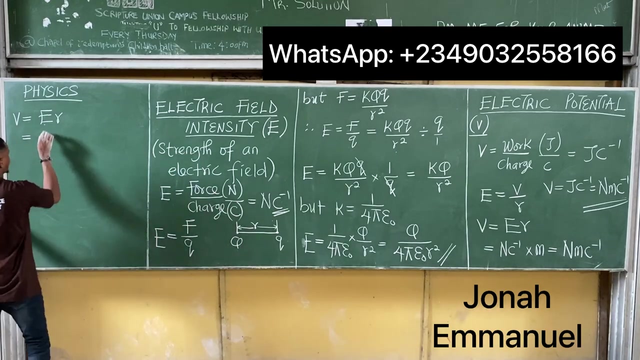 Electric potential. Let us dive Deeper Into Electric Potential. Alright, If we dive deep Into Electric potential, Let us get a formula for it. We said Electric potential V Is equal to E. Times, R Electric field, Times distance Electric field From here. We said Is equal to Q. This is: 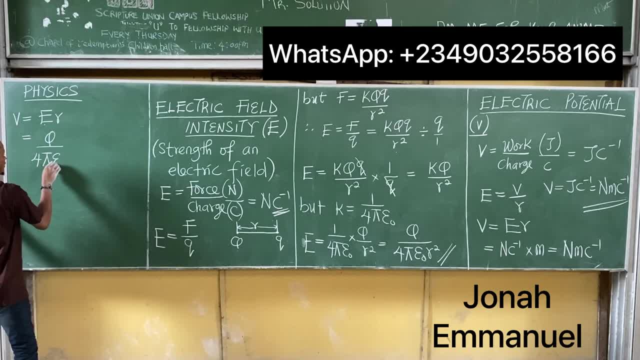 Q All over 4 Pi E naught R square As I have here. This Will now multiply R. That is just So. electric potential V Is equal to From here. Distance R Will cancel One R here. That becomes Q. All over 4 Pi E naught R. 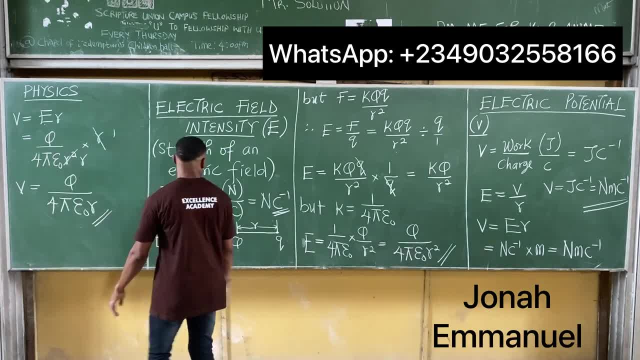 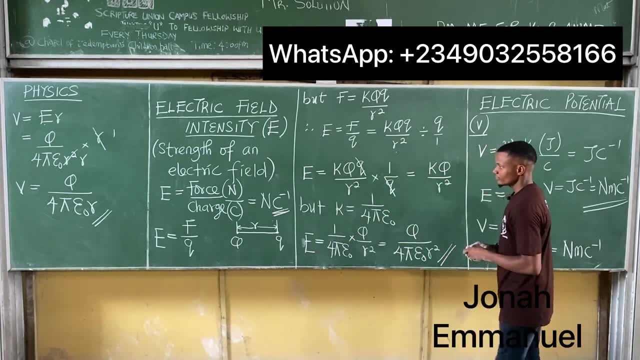 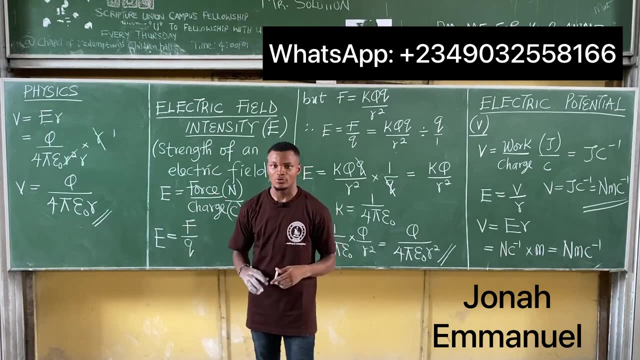 So this becomes The formula For Calculating The electric potential At any point. That is the formula. So if you look at these, They are very similar. They are very similar. All right, These are the. These are the formula. We will take some examples And work on These, Or each of them. 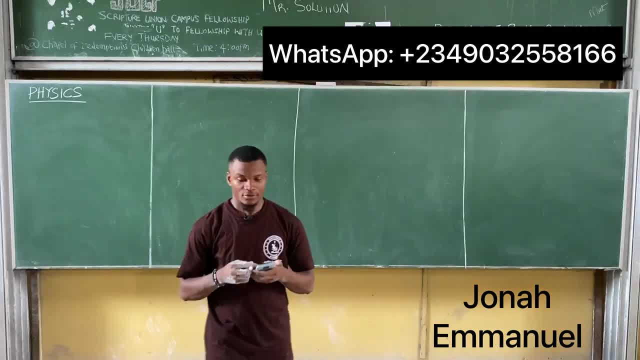 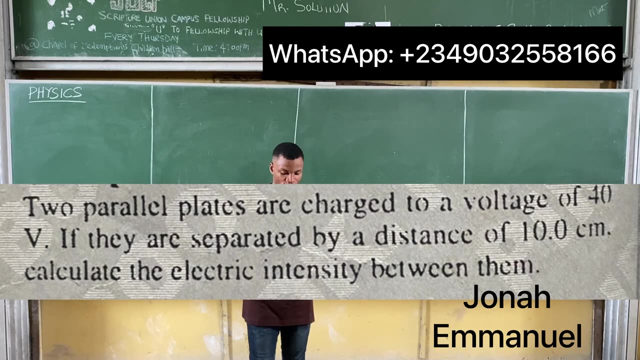 All right. So we will take some examples And solve problems On Electric field, Electric field Intensity. Now, Question 1 says Two parallel plates Are charged To a voltage Of 20 volts, Of 40 volts. If there are Two parallel plates That are charged To a voltage, 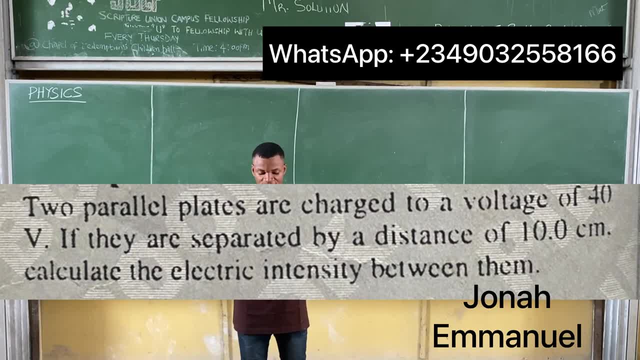 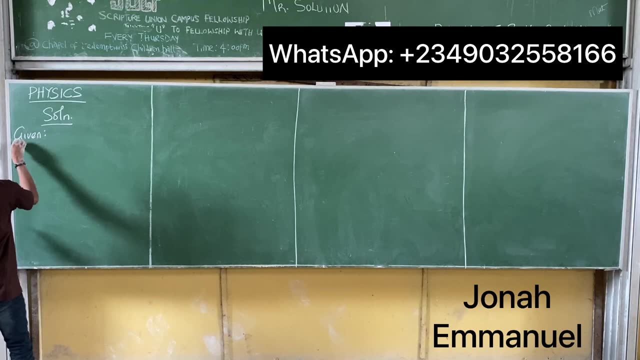 Of 20 volts, Of 20 volts That are separated By a distance Of 10 centimeters, Calculate The electric Intensity Between Them. To solution Um, Case 1: List out, Give parameters. So they said The voltage By 1. I am giving Voltage V As Equal. 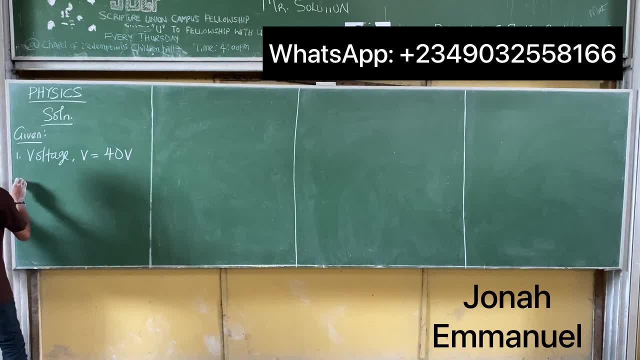 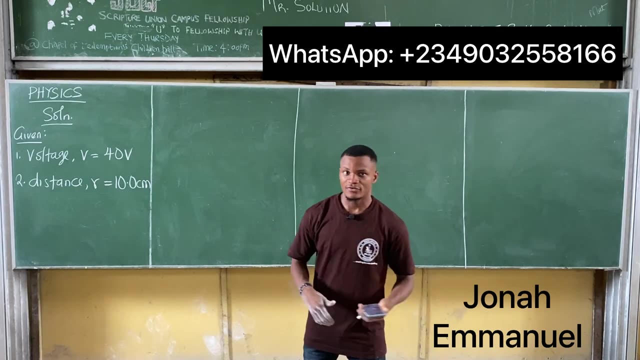 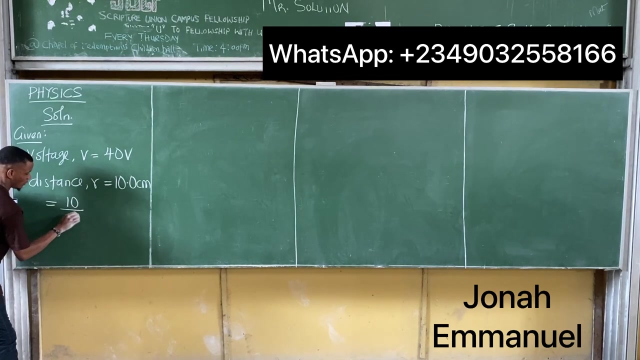 To 40 volts. They said They are separated To By distance, So I am giving Distance I As equal To 10.0 cm. Now My task Is simple: Convert distance From Centimeters To meters, And that will Convert it By 100. That's equal To 10. 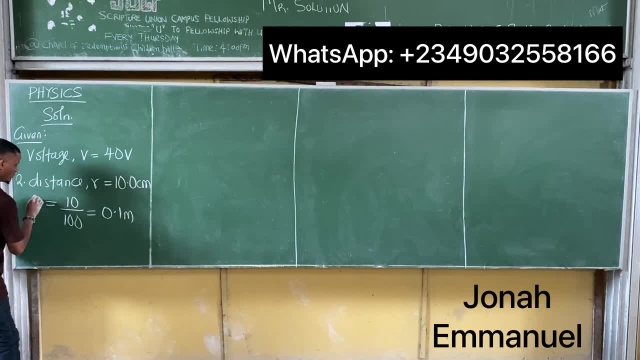 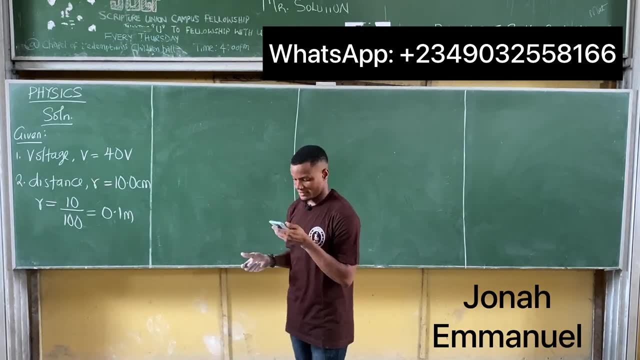 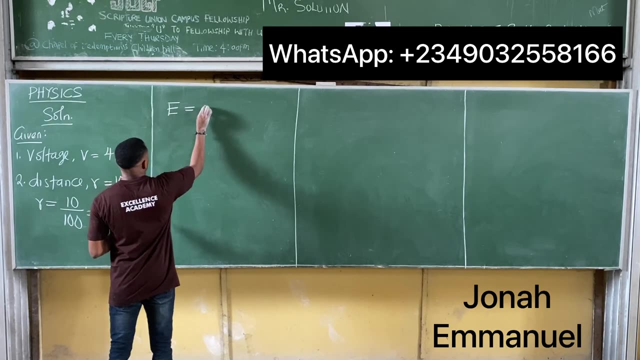 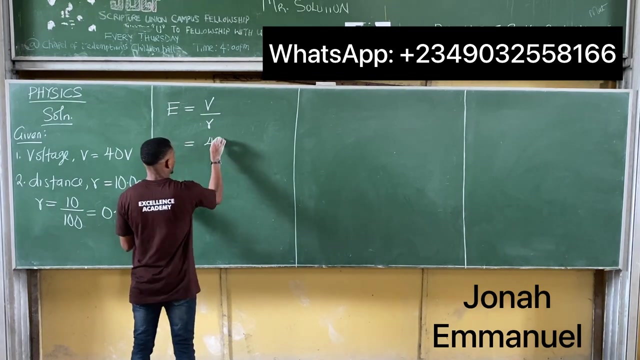 All over 100, That's equal To 0.1 Meters By hours. All right, We have to find, Find The electric Intensity. So we said Let's Keep The intensity. That's. E Is equal To V. All over R, That's equal To. I have this. 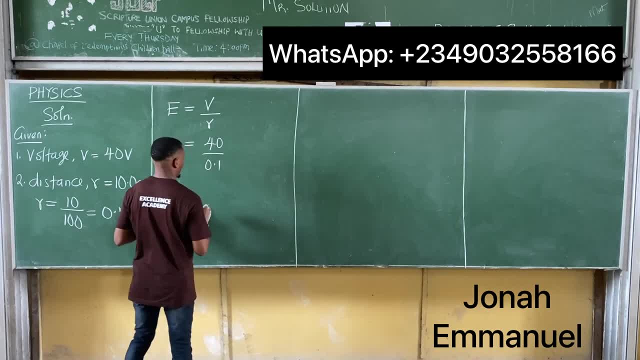 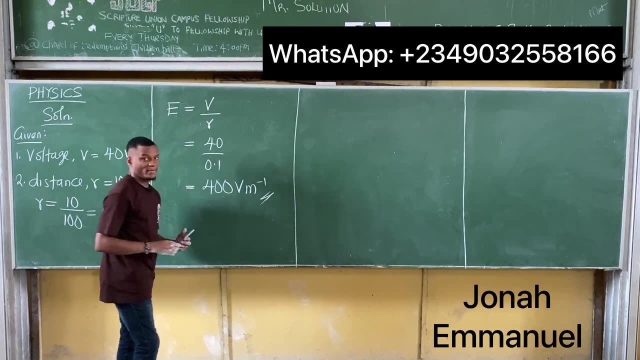 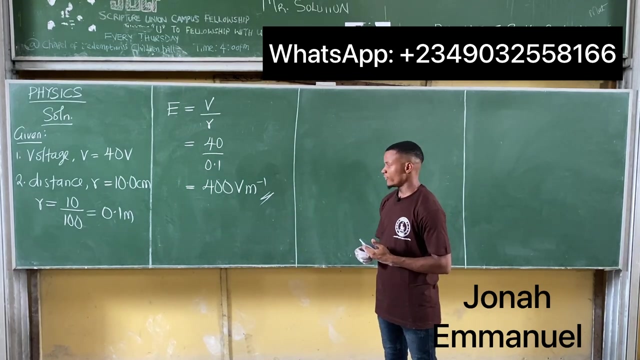 As V Is 40 All over, R Is 0.1. When Converted, The voltage Gives you 400. This Is measured. That's equal To 400 Meters Volt Per Meter As An alternative, SIE To Electric Field. All right, Yeah, So 400 volts Per 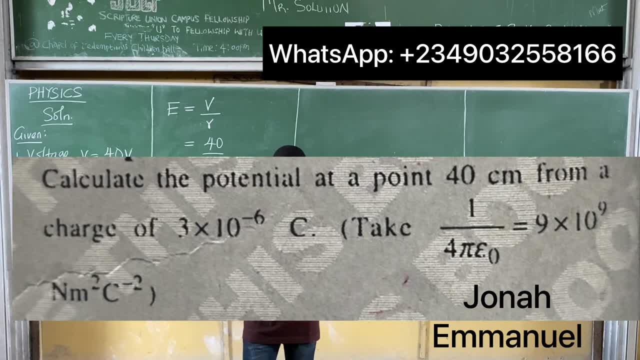 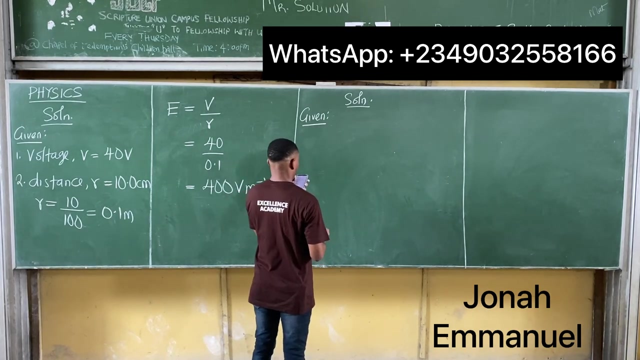 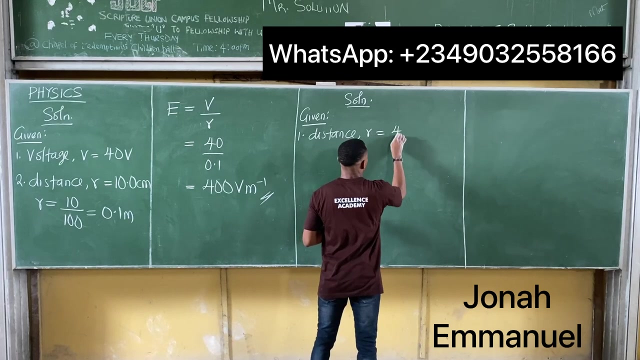 Meter. All right, Let's Proceed. Another Question Here Says Calculate The Potential At The Point 40 As Three Micropole. Take One Of Our Five Inputs As Nine Times Number Nine Newton Meters. Perfect, All right, Simply Enough. Just We Start Parameters In The Point Forty Cent. 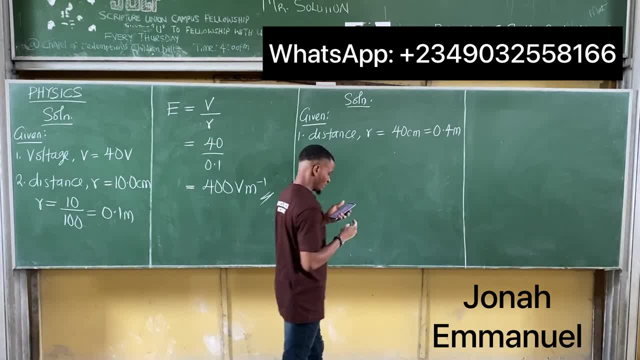 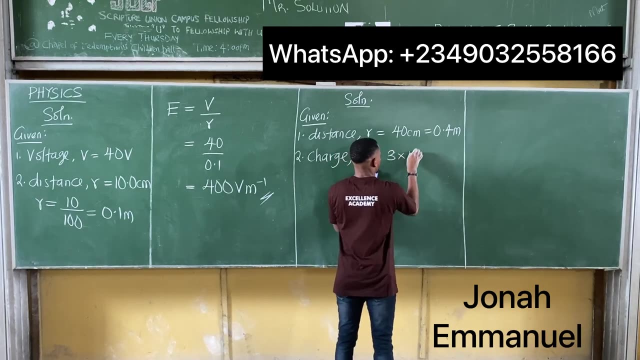 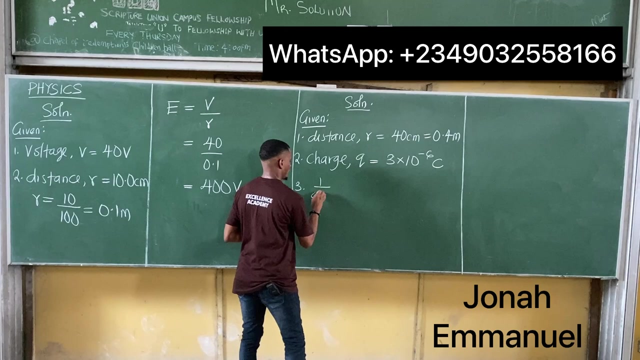 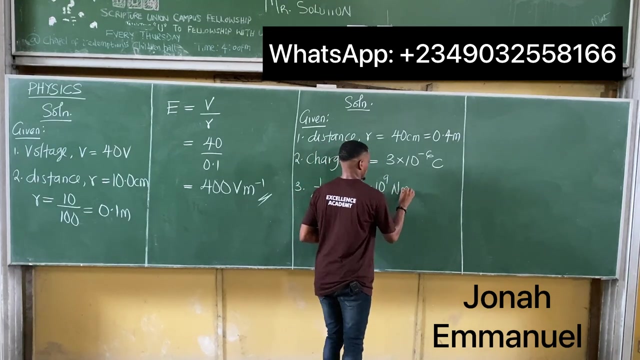 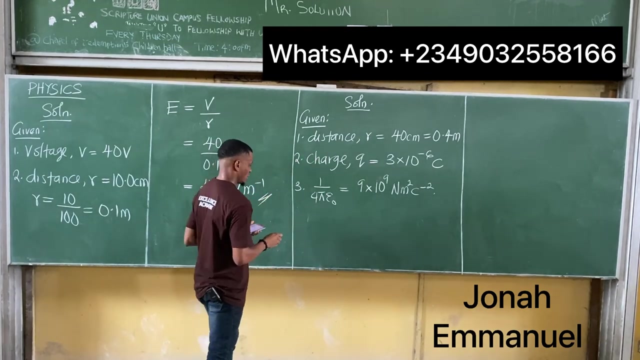 Zero, Four Meters. That's My Best Messages From A Chart. But Soon I'm Giving The Chart Chart That's Q Has Been Three Times Minus. Also We're Giving One Over Four, Five One Newton Meters Square, Square. All Right, We Have To Find The Electric. 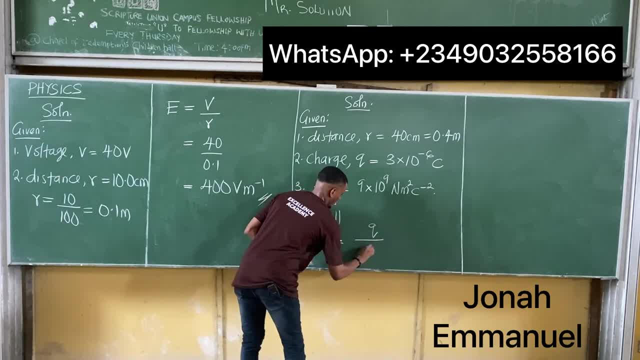 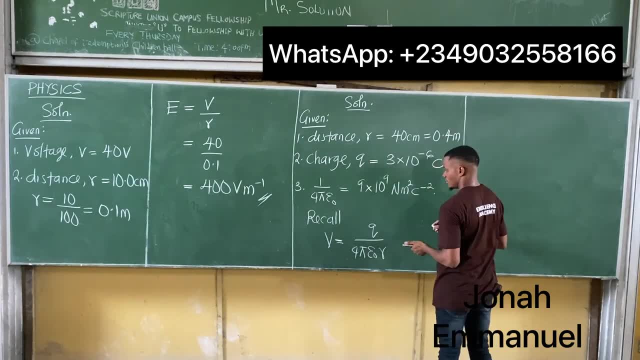 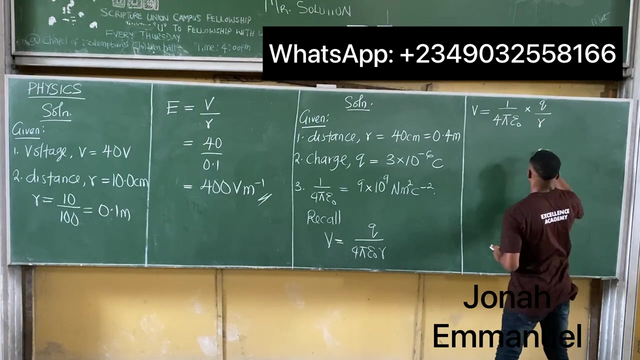 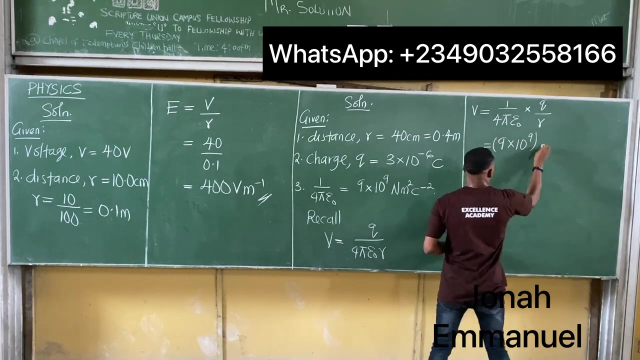 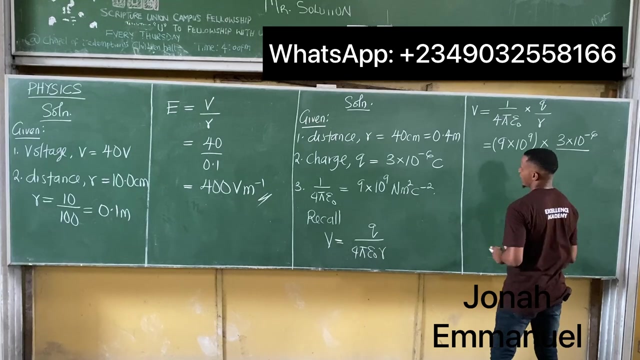 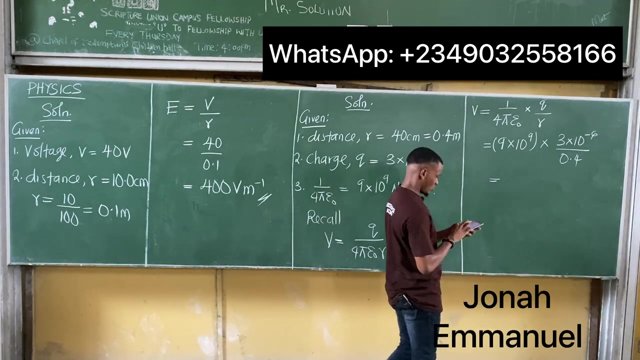 Potential, So We Call The Electric Potential. V Is Equals To Q One Over Four. Five In Times Q All Over R, And That's Equals To This Value, Is Nine Times Ten, Five, Nine Times Q. Q Is Three Times Ten, Five Minus Six All Over. Just Like I.